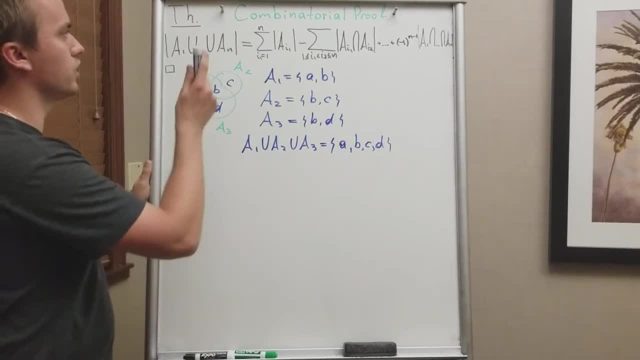 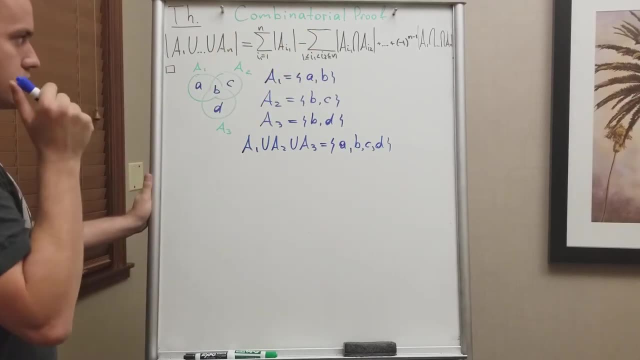 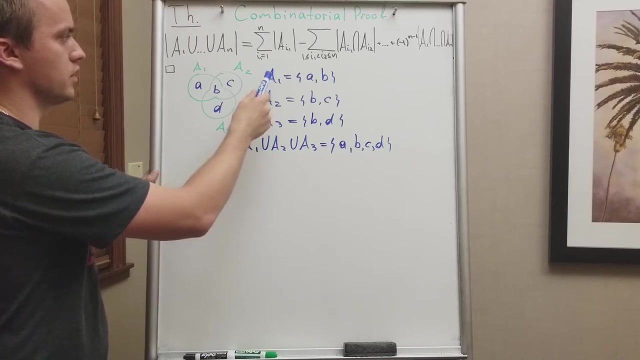 Hello guys, In this video I want to prove inclusion-exclusion theorem by using combinatorial proof. So let's start. Let me show you the idea of the proof. considering this example, I have three different find sets: a1, a2 and a3.. 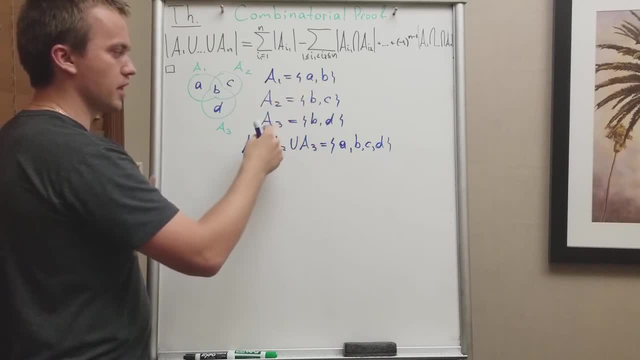 And a1 has two elements. a2 has two elements and a3 has two elements, And what I know is that b belongs to each of these- a1,, a2 and a3. But if I'm going to take the union of all these three- a1, a2 and a3, b belongs to this union only once. 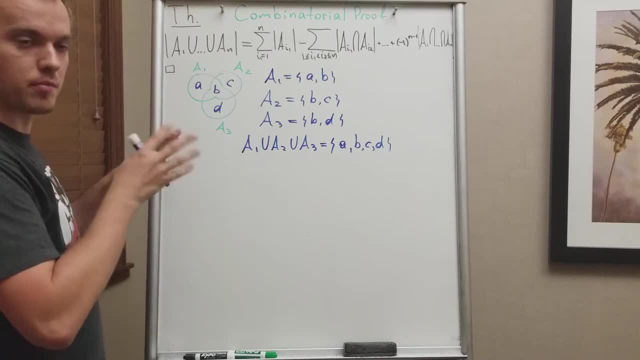 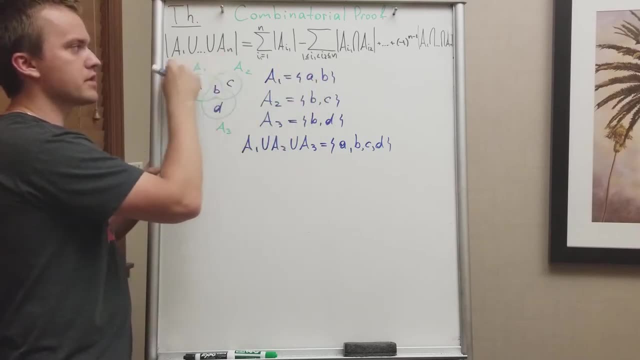 So b doesn't repeat itself. So I want you to remember this idea, this concept: If your a consists of some elements, when you're going to take the union, this element is going to belong to this union only once, once. So when you're going to count these elements, you're going to count them only. 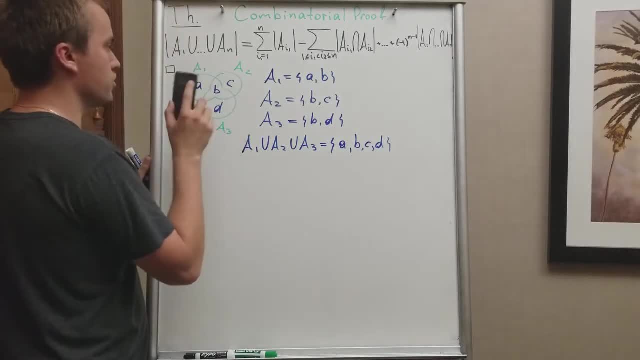 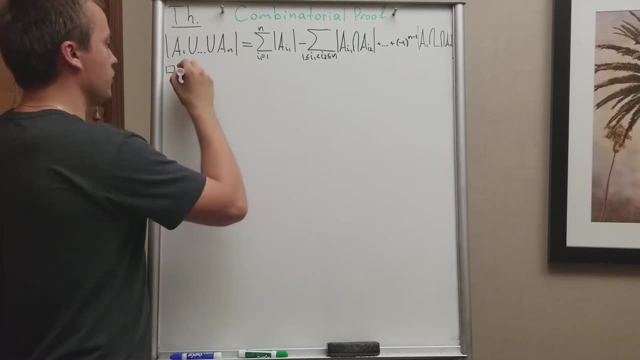 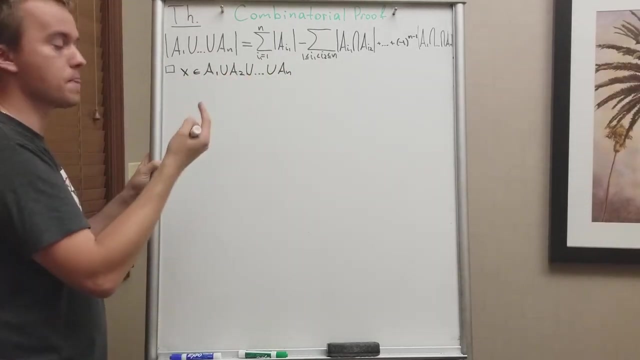 once And how the combinatorial proof actually works. I'm going to erase this. it works in the following way: If we're going to take element x, a1, x belongs to a1, union a2, union a n. We know this x belongs to this union only once. So when we are going to count, 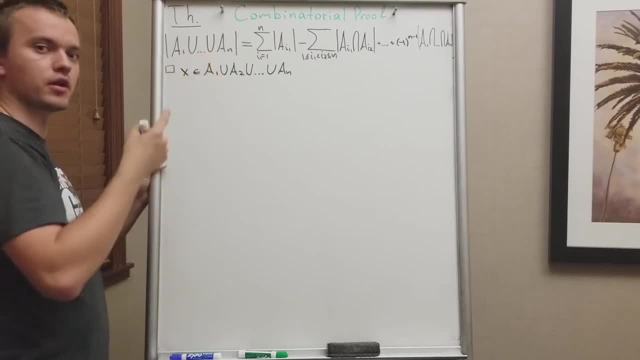 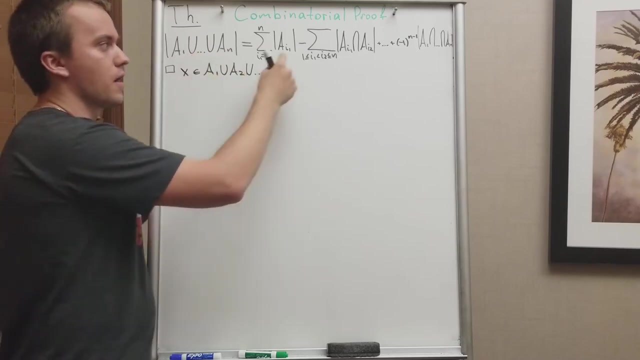 this element on the left-hand side. we're going to count this element only once, But what about right-hand side? So how combinatorial proof works, I'm going to show every time I'm going to choose my element x on the left-hand side if I'm going to count this element on the right-hand. 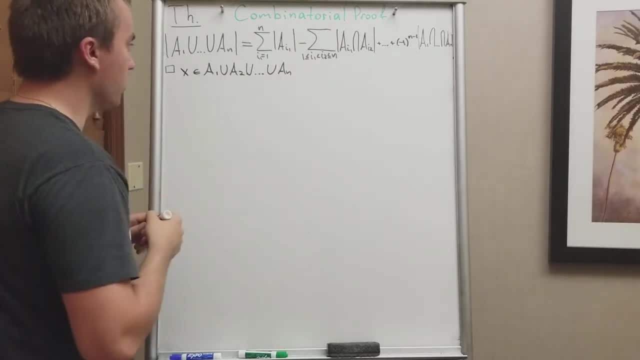 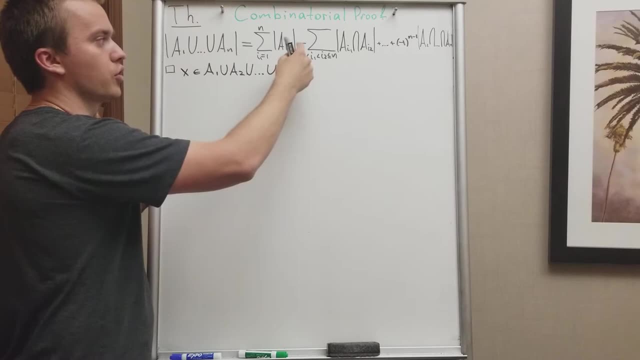 side only once, Because the combinatorial proof works only once. for any of these n But a ginger hand side, I will get 1 as a result. Ok, so this is the idea of the Combinatorial Proof. Again, I'm taking an element on the left hand side and I want to show when I'm going to 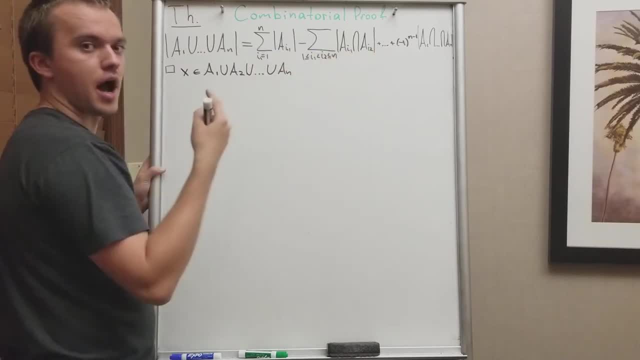 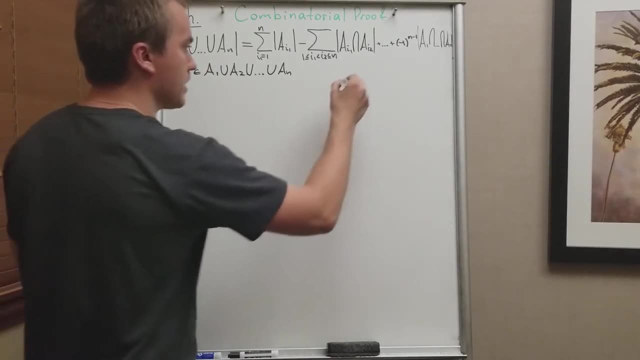 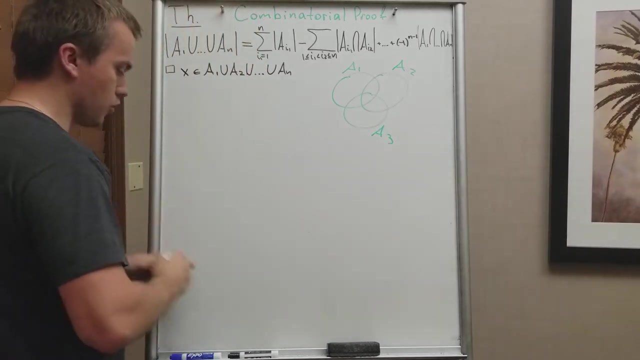 count this element by using this formula on the right hand side, I will get exactly 1.. Ok, so let's consider some example Again. we have, for example, 3 sets: a1, a2 and a3. So if I know that my set x belongs to this union, I can say that my x belongs to some. 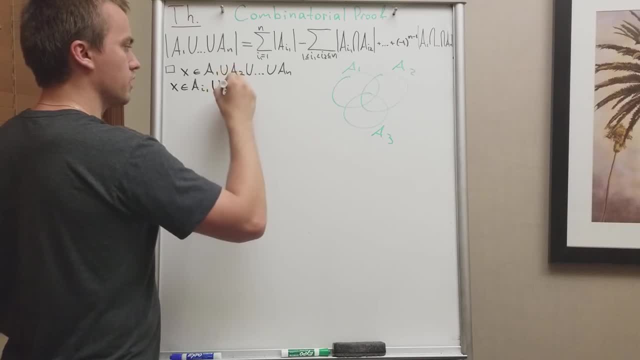 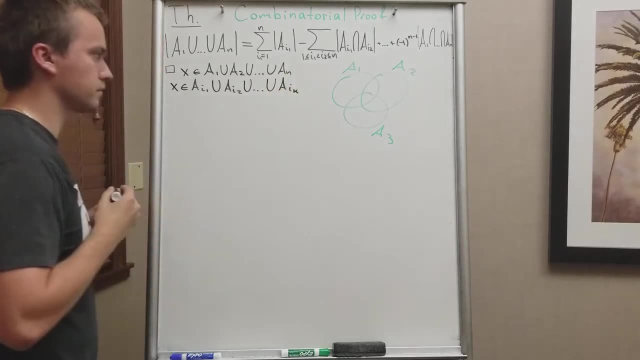 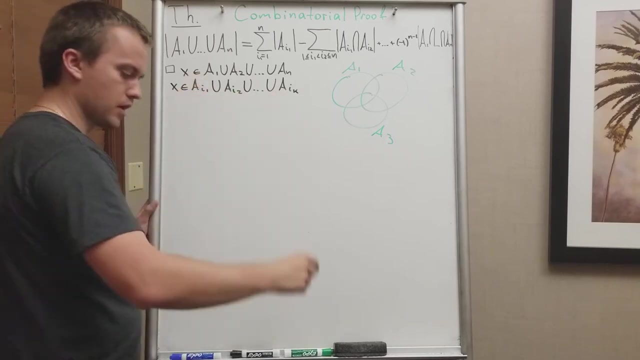 a1, i1 union, a, i2 union, up to a, i, k, And I'm saying that x belongs to each of these a's. So, for example, if I have my element x that belongs to a1, I can say that x belongs. 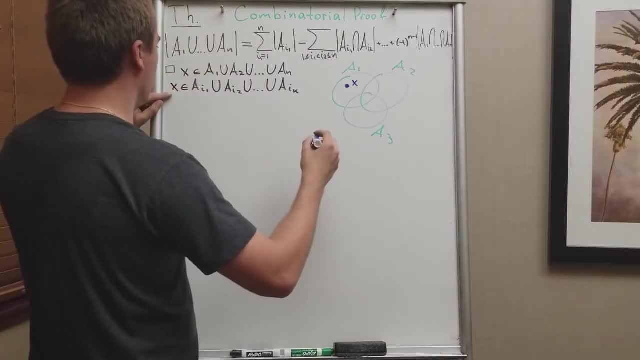 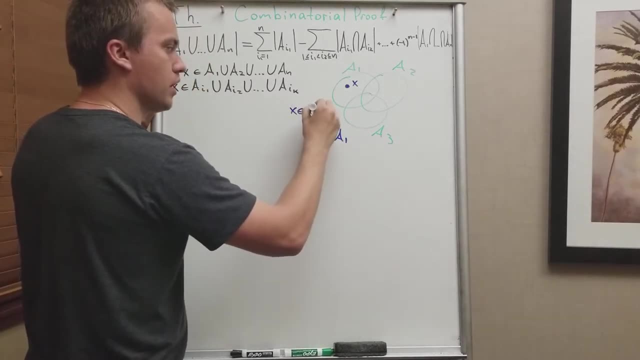 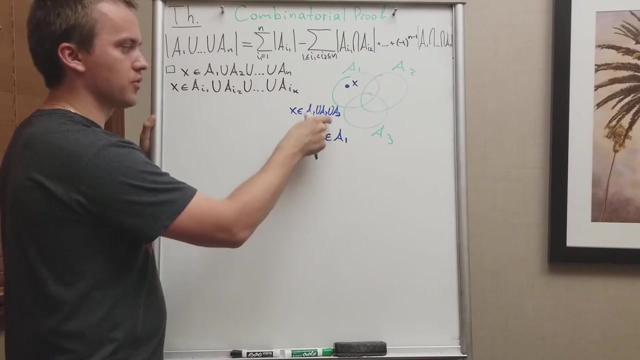 then my second line is going to be just indicate x belongs to a1.. Originally x belongs to a1, union a2, union a3, but I'm taking the subset of this original set only such a's to which my x belongs. 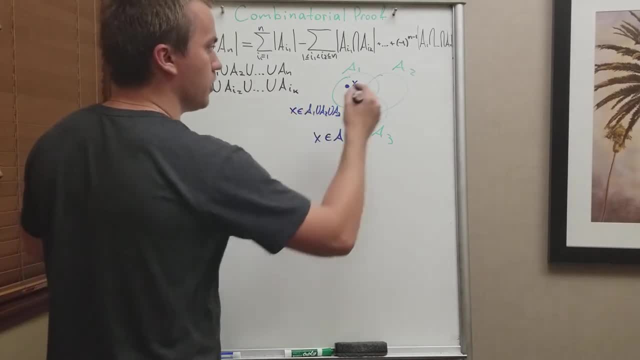 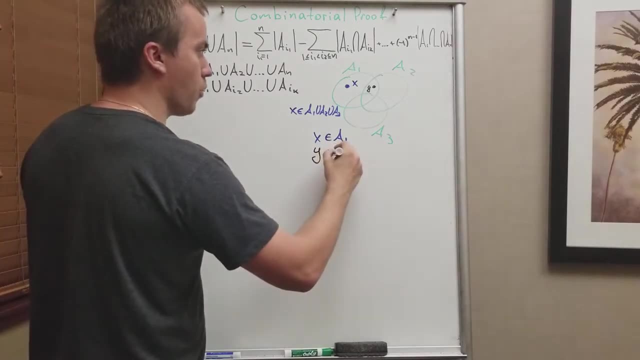 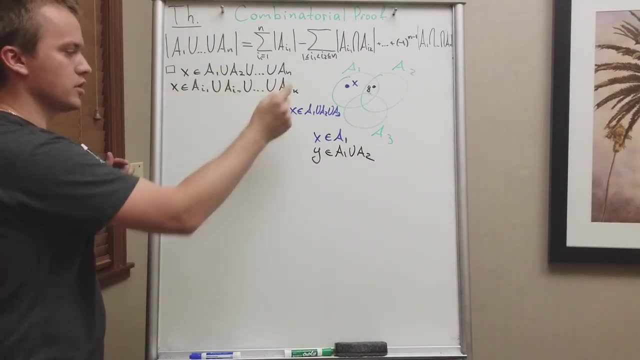 For example, if my x belongs, for example, if I have y, that belongs to a1 and a2, this line means that my y belongs to a1, union a2.. Yeah, so this is the idea. So x belongs to each of these a8s. 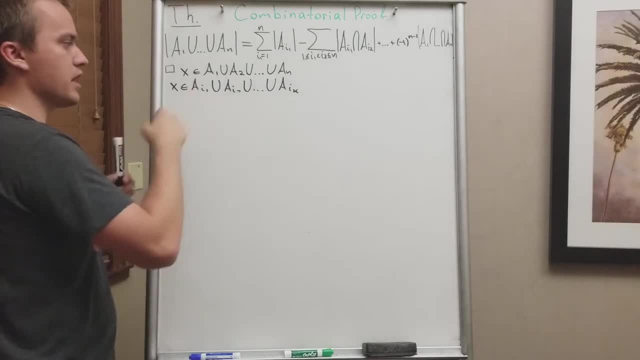 Okay. so what is next After I choose my element? I know the element belongs to each xij, for example: Okay, Okay, Okay. And then let's count how many times I'm going to count my element x on the right-hand side. 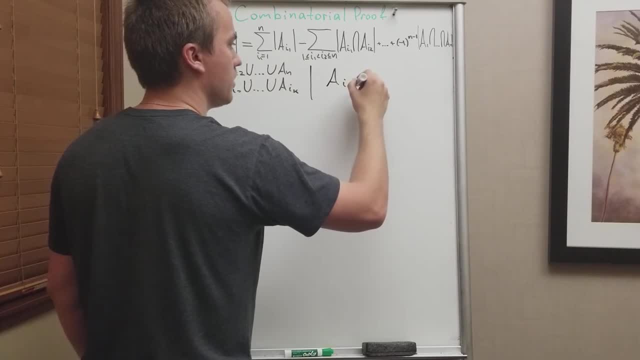 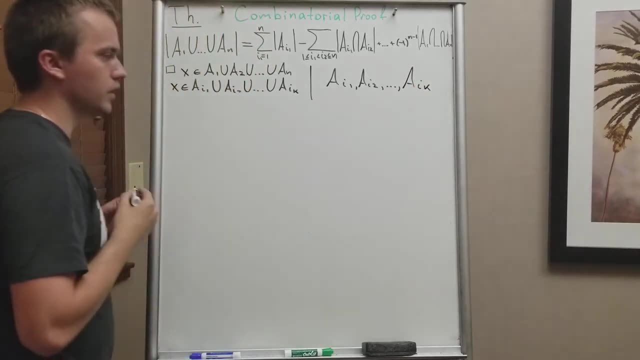 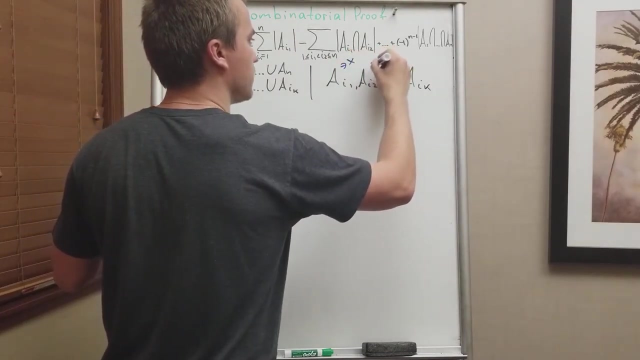 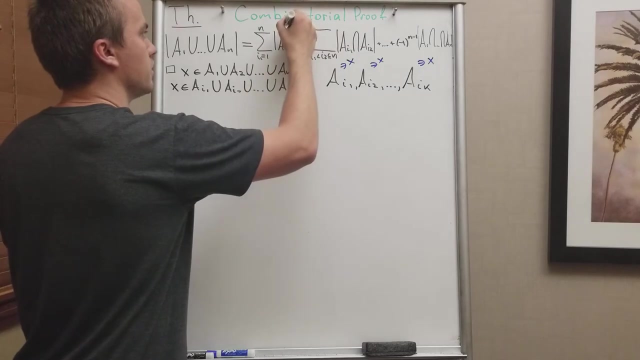 So what I have? I have a1,, a2, and aik, And I know my x belongs to each of this set. And how I'm going to count my element? I'm going to count by using this formula. So how many? if I'm going to use my first term? 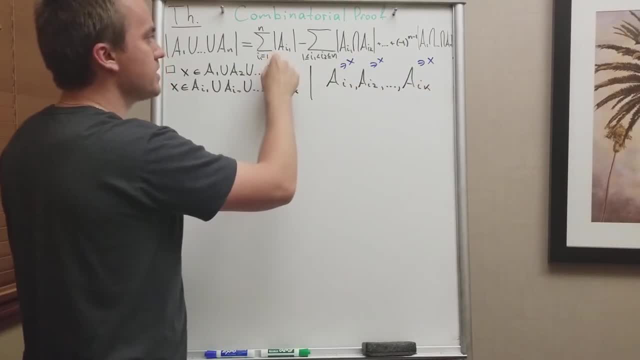 how many times I'm going to count my element x And we can see our x belongs exactly to 1,, 2,, 3, up to k sets. So if I'm going to use my first term, yeah, if I'm going to use my first term. 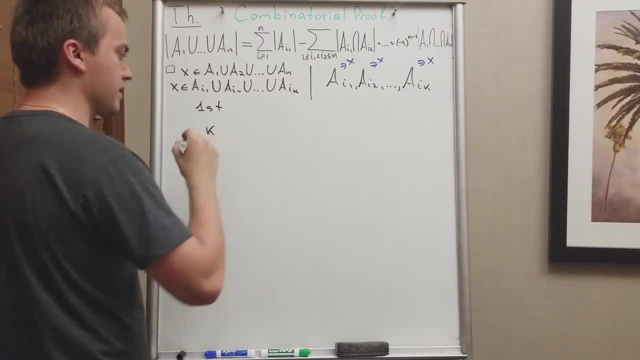 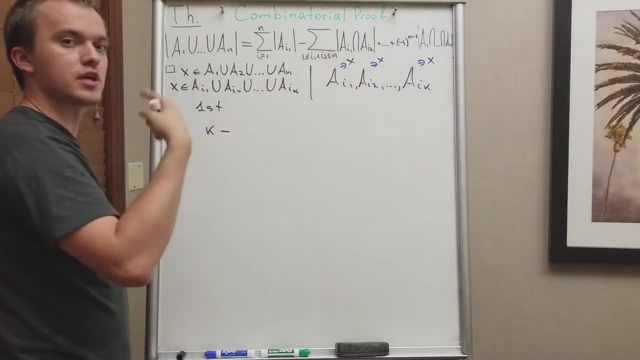 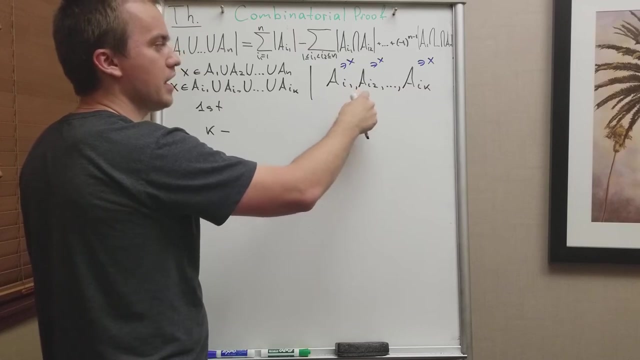 I will get that. I count my element x k times. Okay, what about my second term? For second term, I'm going to subtract the numbers of my k's. But what does it mean, second term? Let's think about this. Second term means x belongs to a1,, x belongs to ai1 and ai2.. 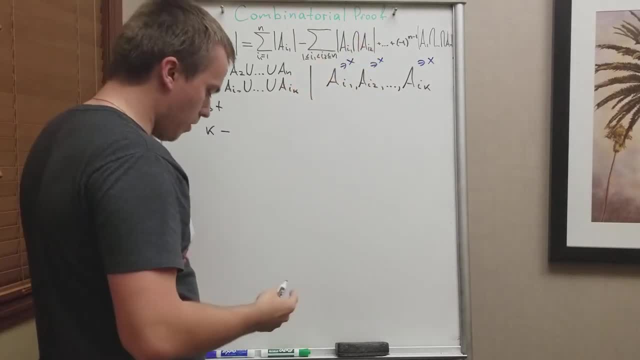 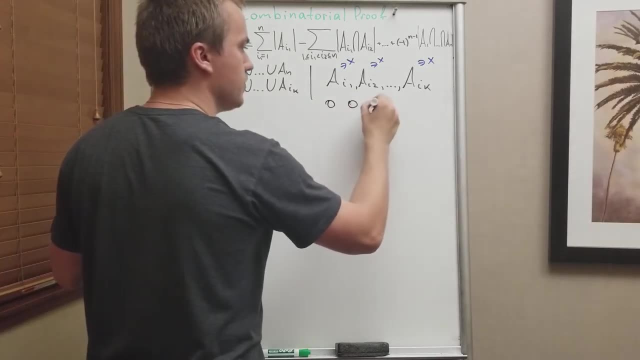 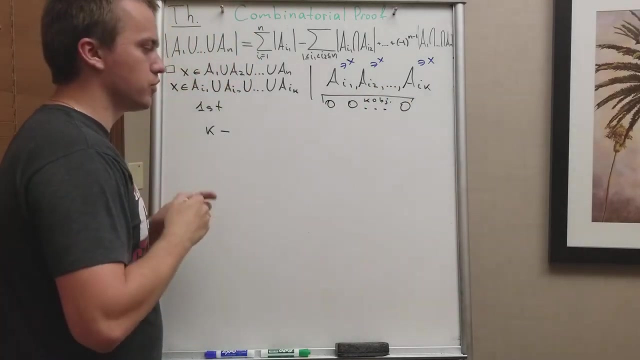 Or what we're doing in this term: among all these k pairs we're choosing two pair. But you can remember from combinatorics, if you have k objects and if you want to choose among these k objects exactly two objects, it's going to be k choose 2.. 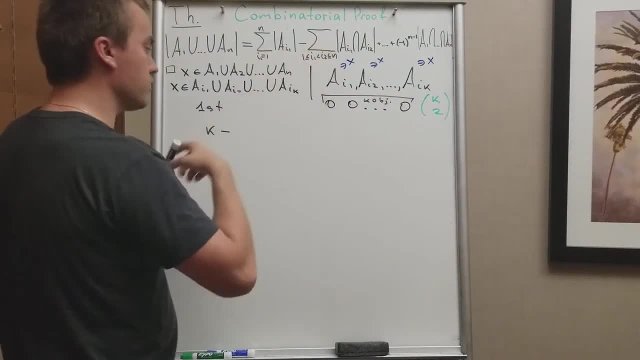 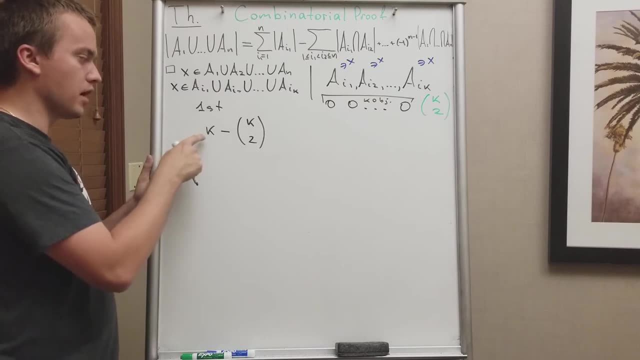 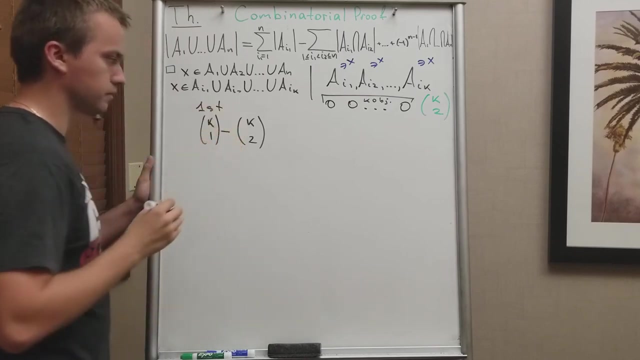 So, actually for our second term, we're going to subtract k choose 2 elements x And again, by using this formula, by using binomial coefficient, you can rewrite your first term as k choose 1.. Okay, what about the third term? 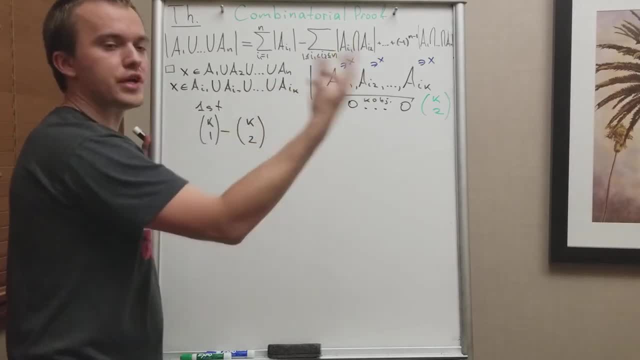 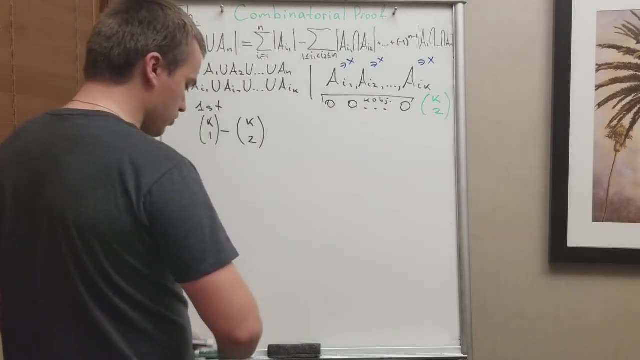 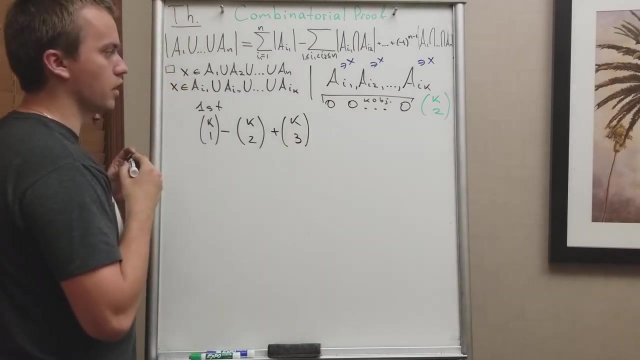 For the third one, we're going to take the intersection of three a's. So among these k objects we're going to choose three circles. And if we're going to choose three circles, we're going to add k. choose 3 terms. 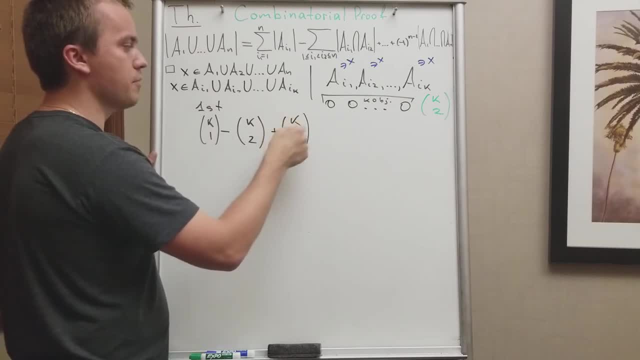 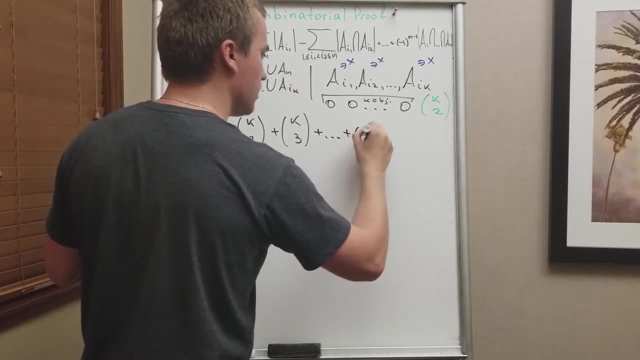 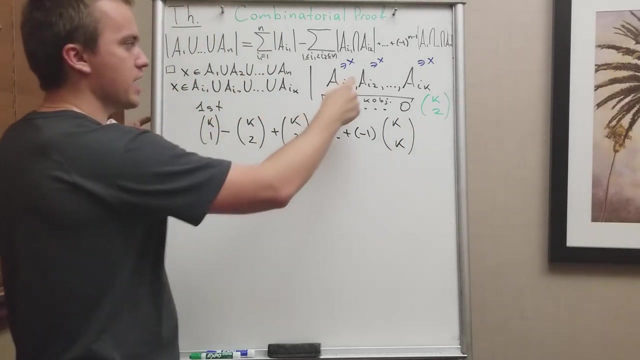 So what does it mean? It means this is exactly number. how many times I'm going to count my x in my third term? And we're going to sum up this until negative 1 to some power. k, choose k Why? Because you know that x belongs to only the subsets of a, so there's only one x which is going to belong to all of them. 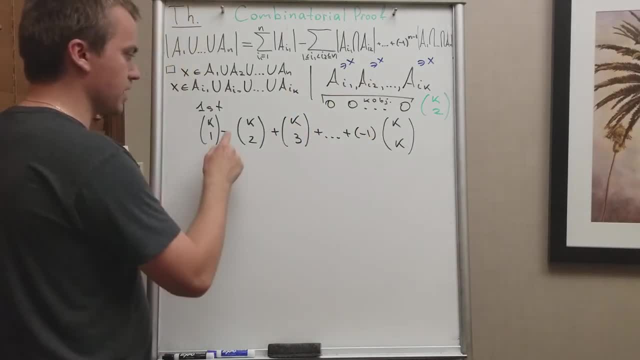 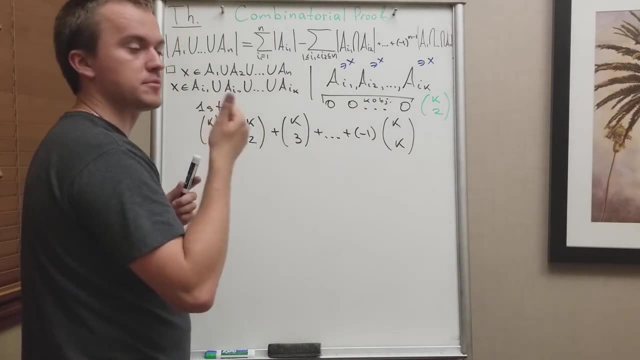 And which power do I need to choose? And I just need to check. I can see that my second term has negative sign. So it means if my k is 2, my power must be odd. So I will write my power as k minus 1.. 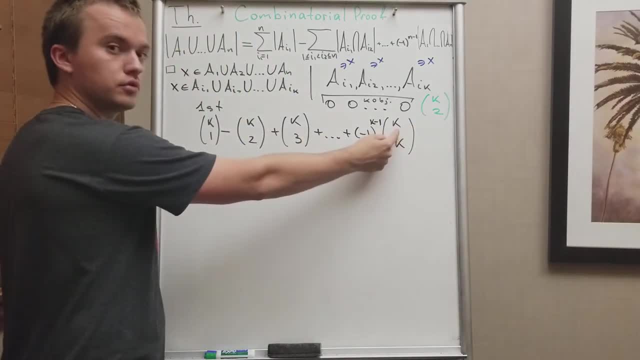 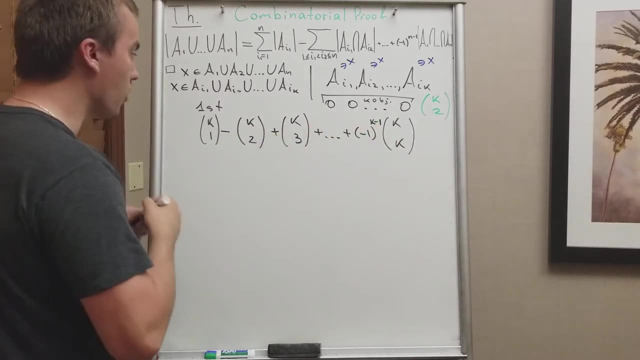 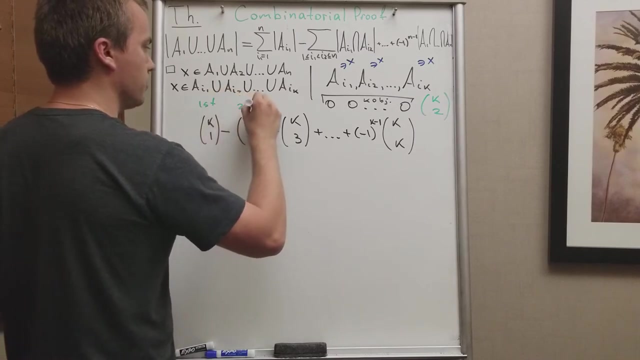 Why? Because when I have k equals to 2, I have 2 choose 2 minus. So I have 2 choose 2 minus because this power is 1.. Okay, and we got this formula. We got that. this is true for first term, second term, third term and this is my kth term. 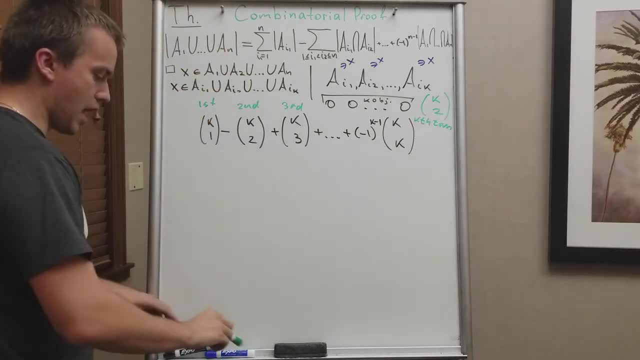 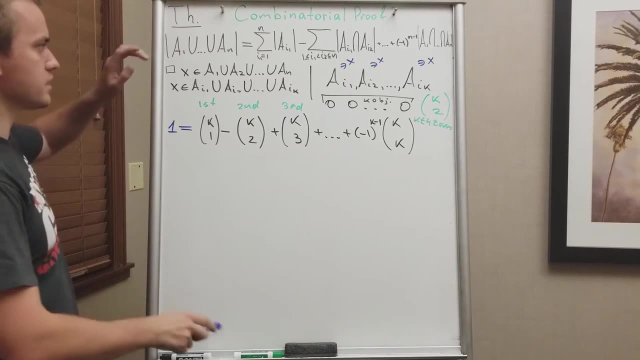 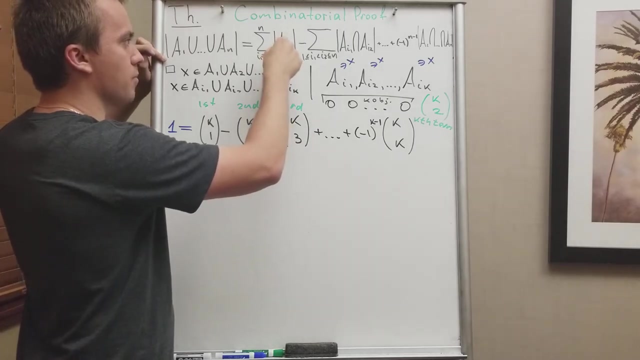 Yeah, And what is our goal? Our goal is to show that this, the whole thing, is, equals to 1. Why? Because we count our elements on the left-hand side only once and we want to show every time in this sum counting my elements. 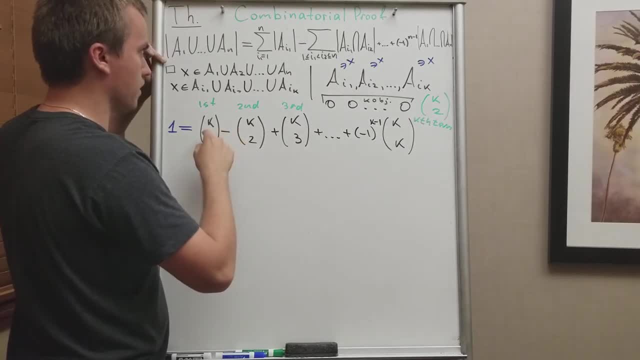 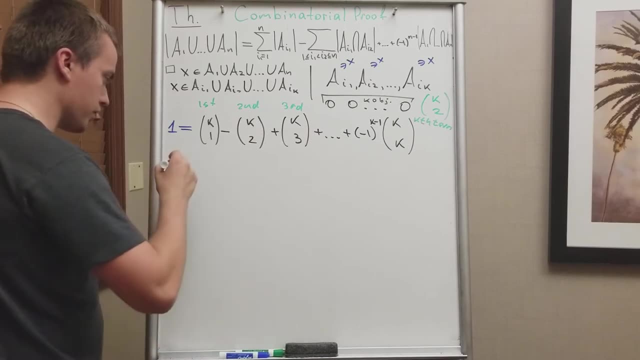 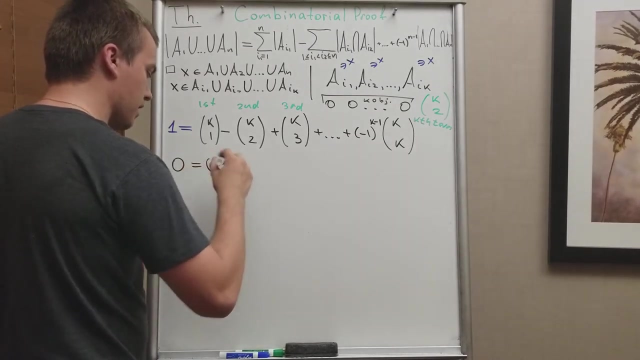 I want to show that how many times we're going to count this element, we're going to add up to 1.. And how are we going to show this? You remember, let's take our 0. We have 0. And what we can do with 0, we can write this: 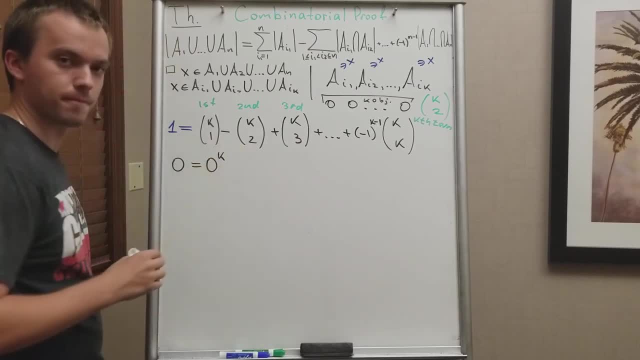 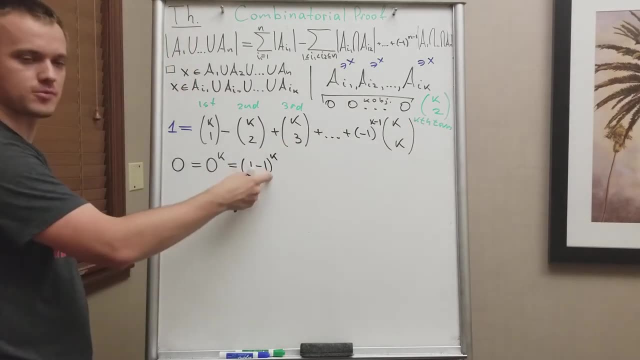 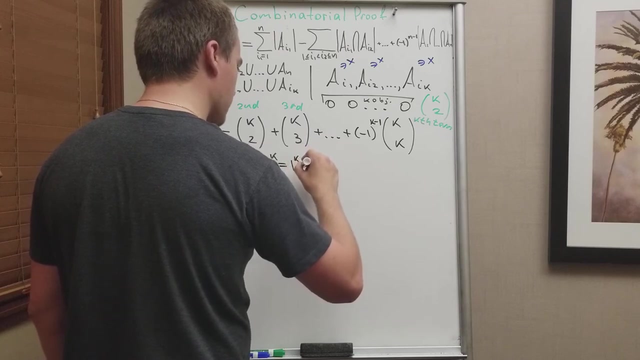 Okay, let's make it fun. We can write this: 0 to the k, Yeah, And 0 to the k is equal 1 minus 1 to the k. So add 1 and subtract 1.. But here, by using binomial theorem, I have 1 to the power of k plus k. choose 1.. 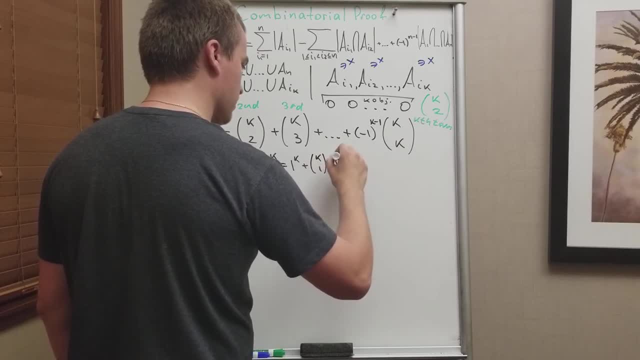 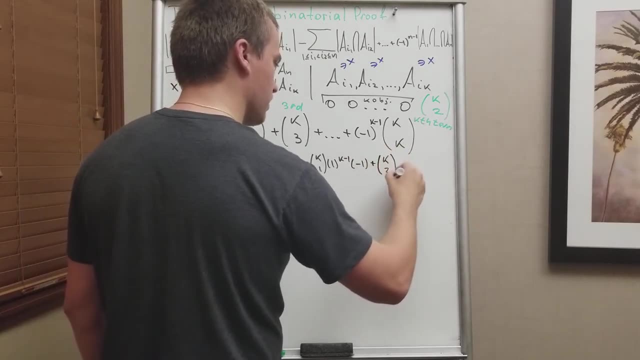 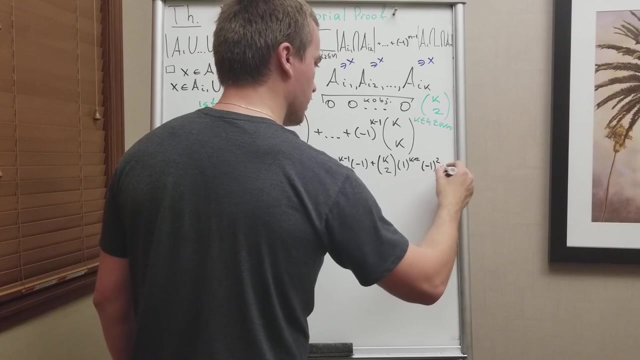 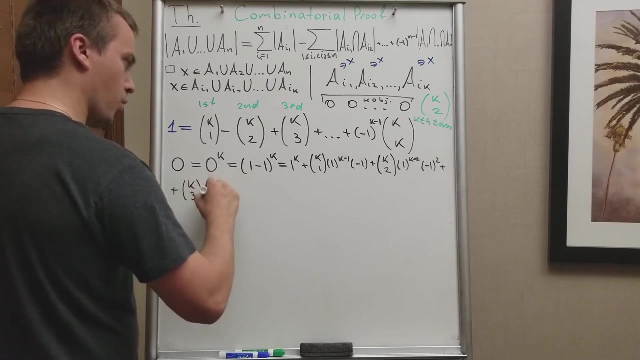 Okay, 1 to the power of k minus 1 minus 1 plus k, choose 2.. 1 k minus 2 minus 1, squared plus k, choose 3.. 1 k minus 3 minus 1 cubed And up to: 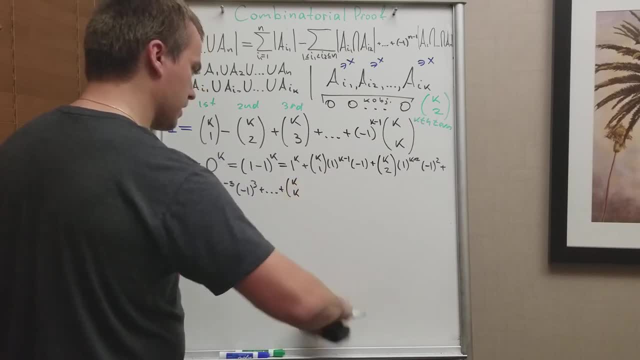 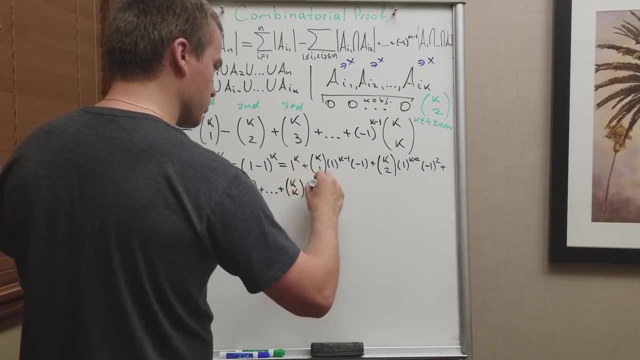 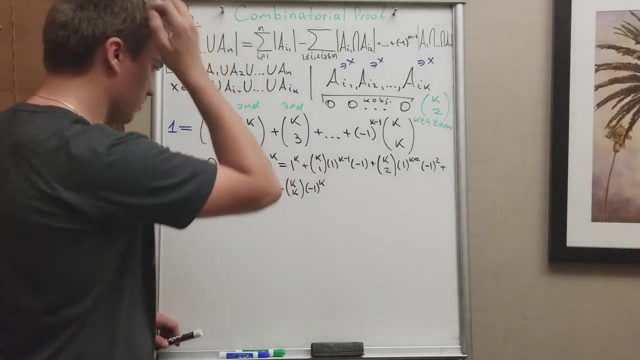 k choose k. And here I don't need to forget about my sign. I will have k choose k up to minus 1 to the k power. Yeah, So here I just use my binomial theorem. I expand this by using binomial theorem. 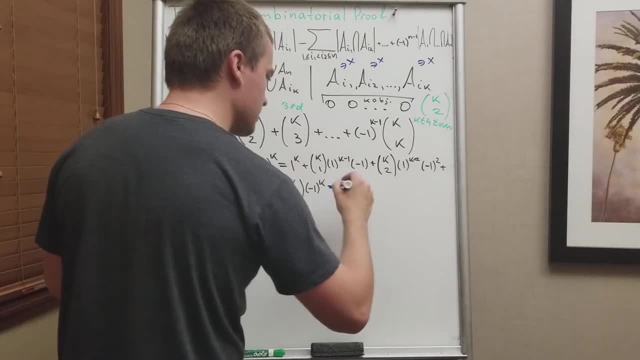 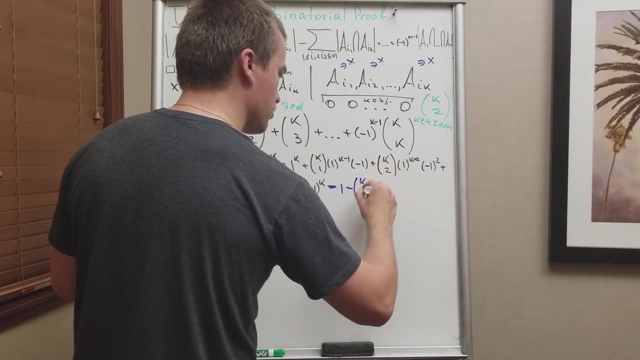 And what I will get As a result. I will get this is going to be equals 1 plus this term going to give me I have minus sign, So minus k choose 1.. k choose 1 plus k choose 2..